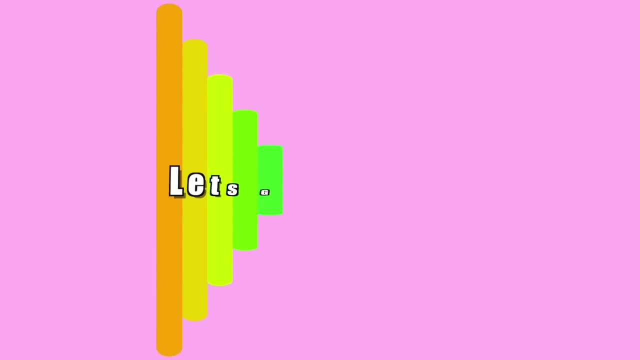 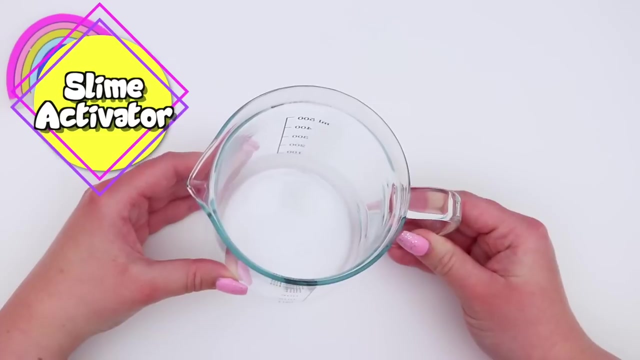 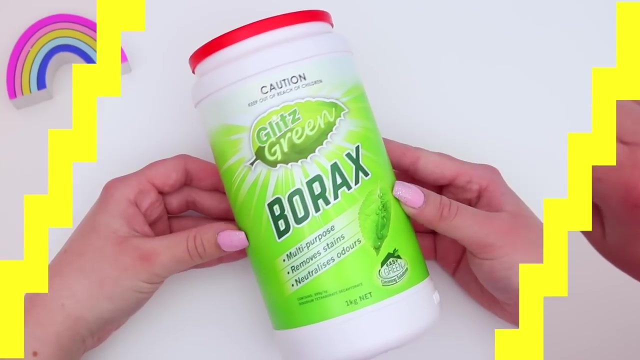 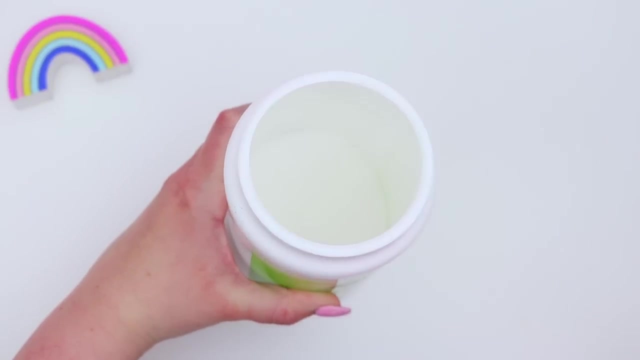 It is so much fun and I am so excited about it. So we're going to start off by making our slime activator, and what activator is is it's basically what's going to make our glue into slime, so it's super important. So to a jug, just add one cup of warm water, and then you're going to need borax- and I just found this in the cleaning aisle of my supermarket- and then just take half a teaspoon of the borax and add this to the water, and then you just want to stir it up. 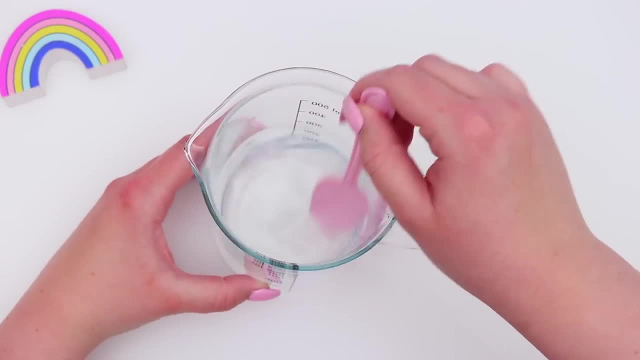 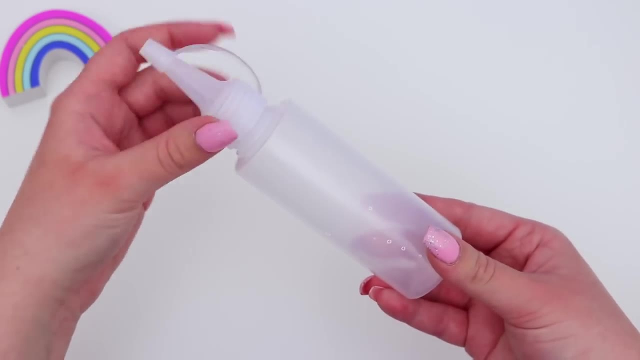 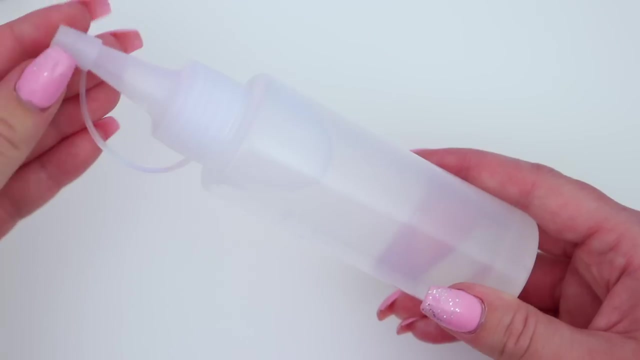 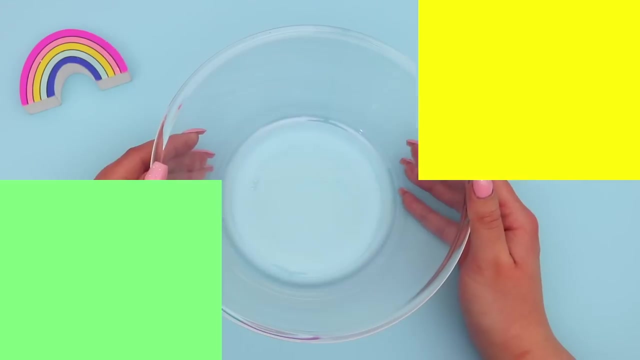 Stir it until all the borax has dissolved. Now you can leave your slime activator in the jug, but what I've been loving doing lately is actually adding it to a squeezy bottle like the one you can see here. So I'm just carefully pouring it into the bottle and then popping the lid back on, and I just love using this squeezy bottle to add my slime activator to my slime, and I just popped a label on it here just so everyone knew that it was activator. So now it's time to make our slime. So you're first going to need a bowl and then you're going to need some peaches. 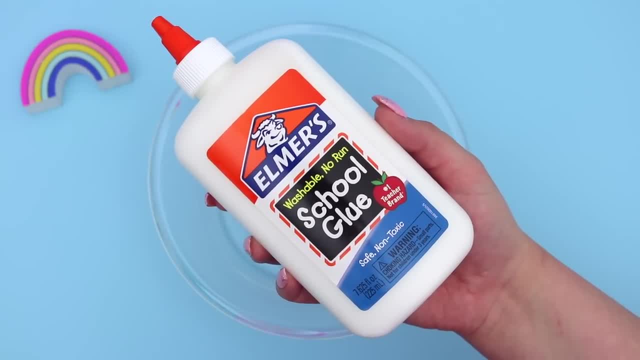 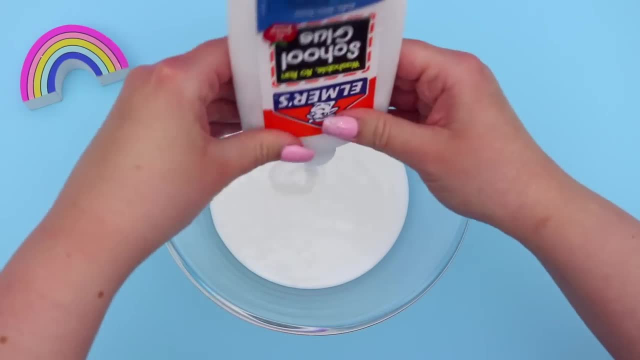 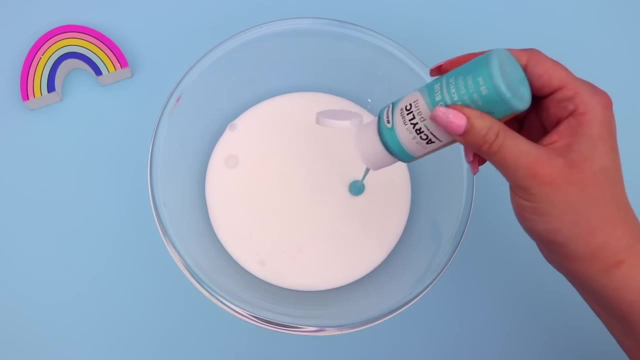 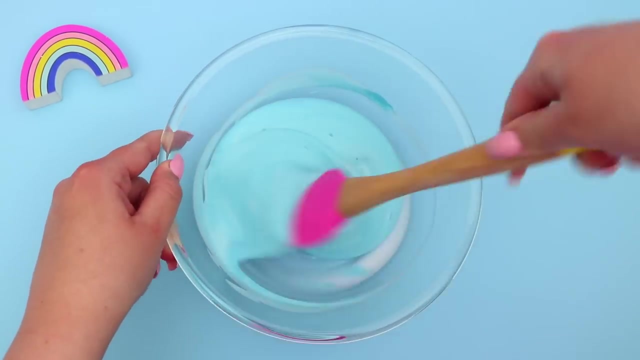 So I'm just going to take some UVA school glue and just add a bottle of this to the bowl. So I'm using Elmer's school glue. that's just my favourite one. Now, this is an optional step, but I love colouring my slime. I love making them really bright, fun colours, and you can either use acrylic paint or you can use food dye. I'm using acrylic paint here, so I'm just adding a little bit to the glue and then mixing it in until it's all the same consistency. 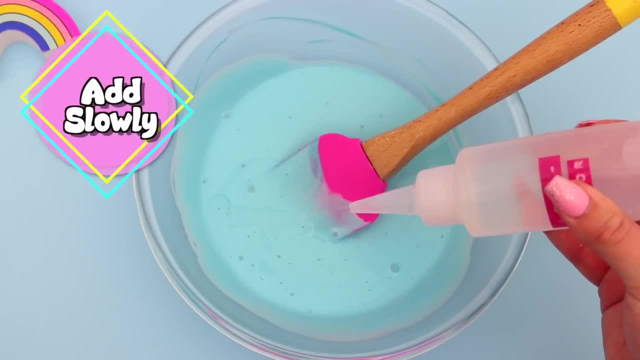 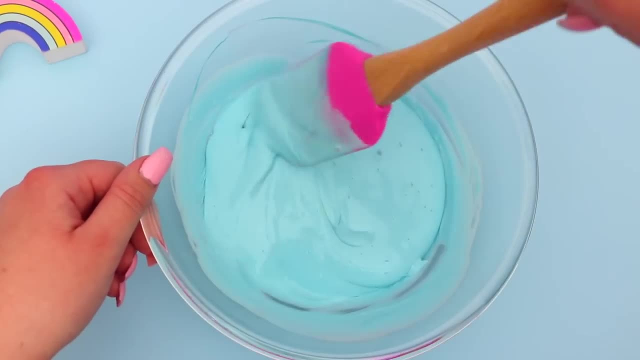 Now grabbing that activator that we prepared earlier. Just squeeze in a little bit of this at a time. You're not going to need that much. I know we've prepared like a bigger batch of it, but you're only going to use a tiny amount. 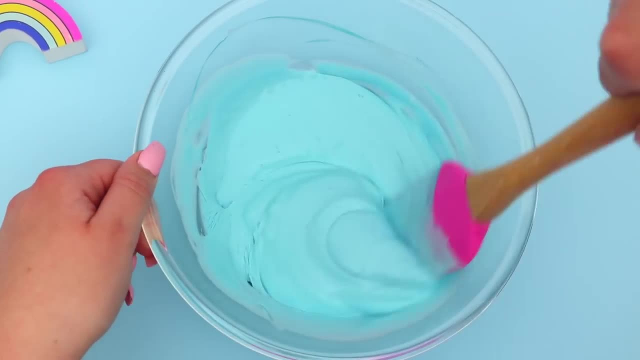 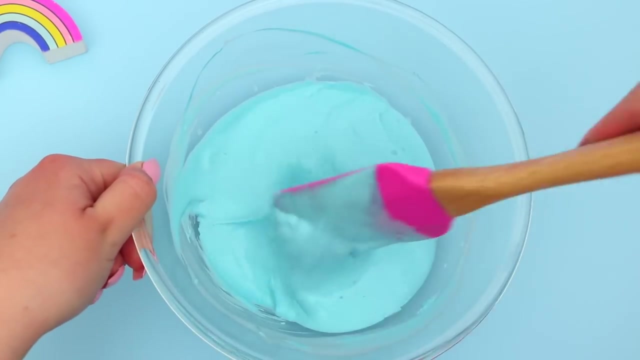 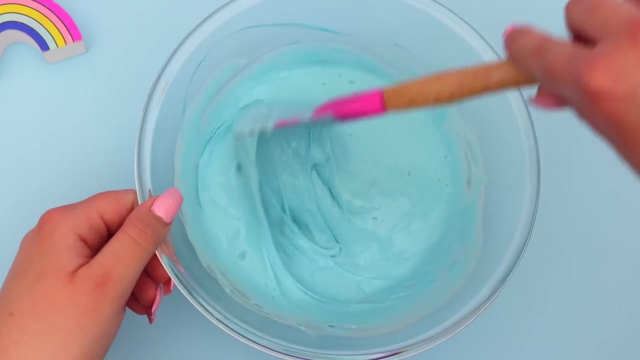 So just squeeze a little bit of the activator into the glue mixture and start mixing it, and immediately you'll see that it's starting to form a slime texture. So you just want to continue stirring it super slowly and you also want to make sure that you're adding your activator very slowly because you don't want to over activate your slime, because then it will be super rubbery and not stretchy at all.